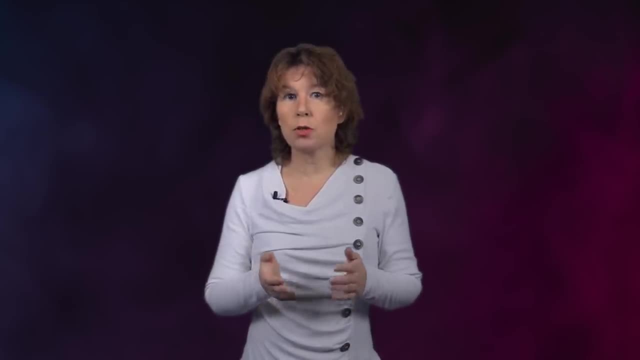 If you want to solve equations like this, you therefore introduce a new number, usually denoted i, with the property that it squares to minus 1.. Interestingly enough, just giving a name to this equation is not the problem. Just reduce the number and, of course, the real numbers. But if you don't, then you have to prove it's true. 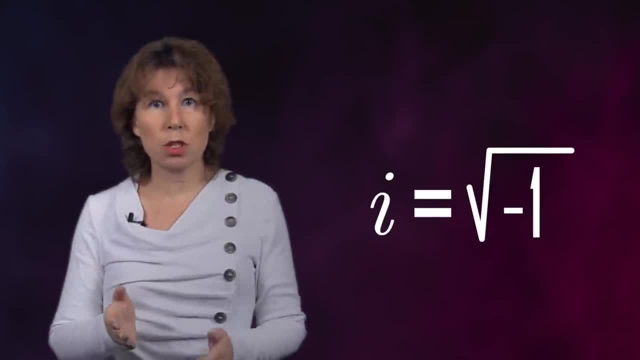 What is the same for a real number? They are just small numbers in the form of individuals like pi. Interestingly enough, just giving a name to the solution of this one equation and adding it to the set of real numbers turns out to be sufficient to make all algebraic equations. 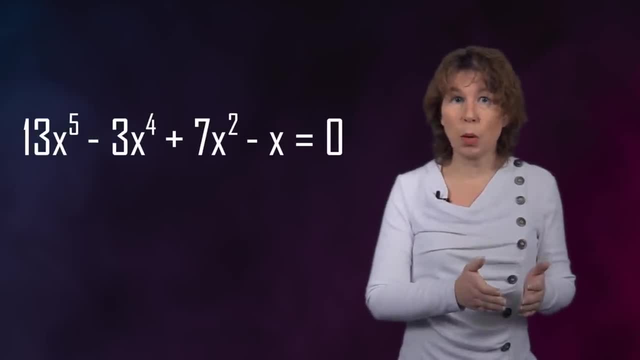 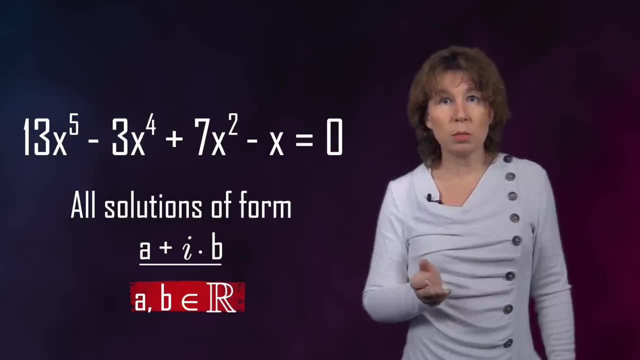 solvable. Doesn't matter how long or how complicated the equation, you can always write all their solutions as a plus i, b, where a and b are real numbers. Fun fact, this doesn't work for numbers that have infinitely many digits before the point. 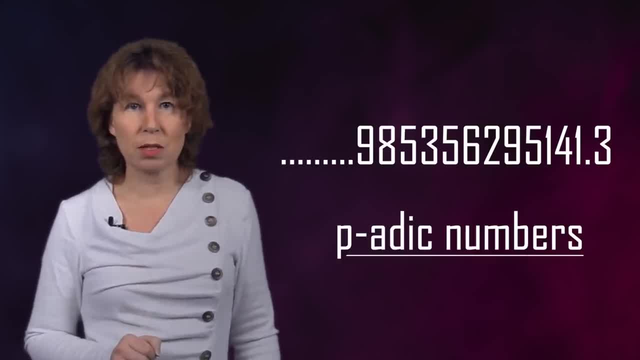 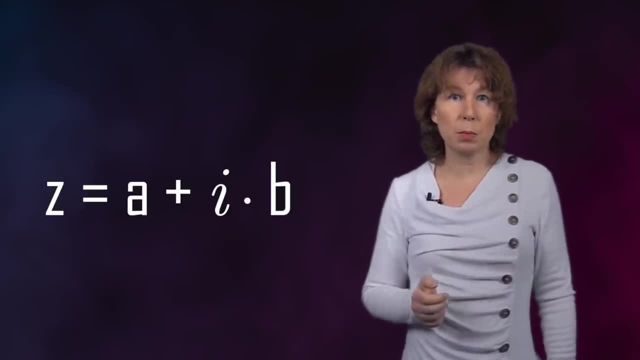 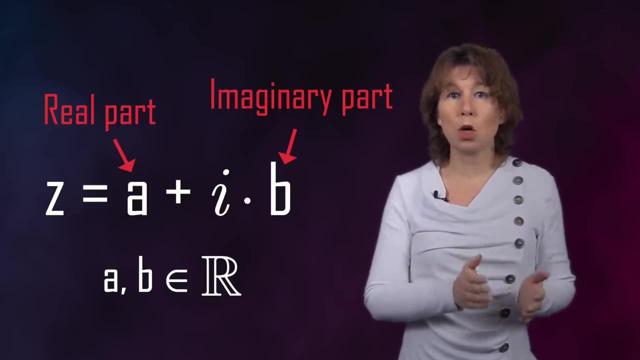 Yes, that's a thing. They are called periodic numbers. Maybe we'll talk about this some other time. Complex numbers are now all numbers of the type a plus i times b, where a and b are real numbers, A is called the real part and b the imaginary part of the complex number. 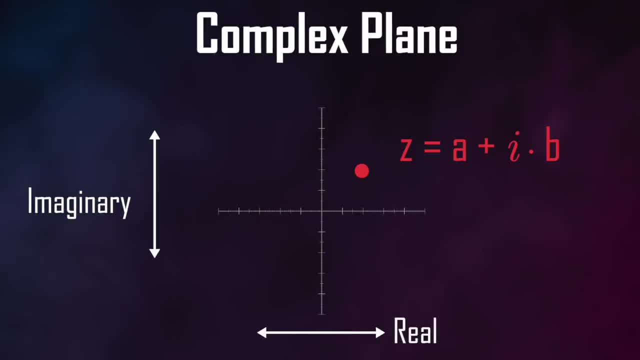 Complex numbers are frequently drawn in a plane called the complex plane, where the horizontal axis is the real part and the vertical axis is the imaginary part. I, at the end of this video, will show you how to do this. I, at the end of this video, will show you how to do this. 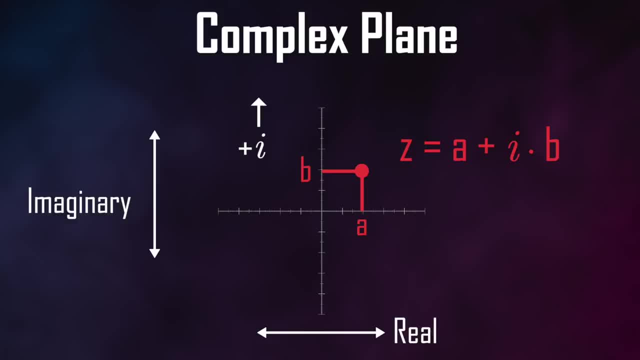 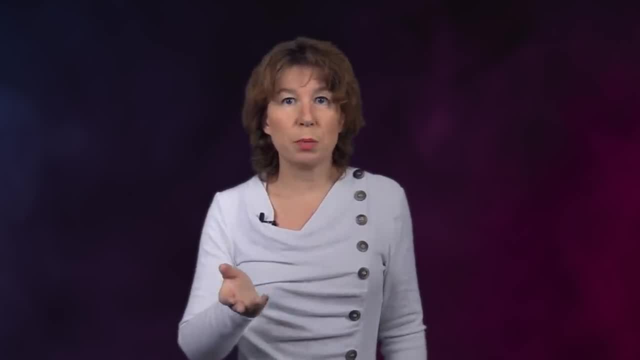 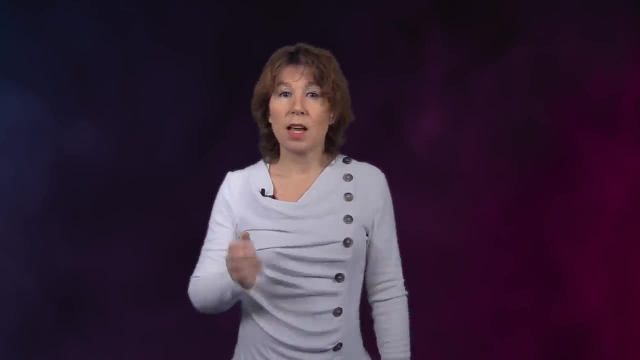 But this looks the same as if you draw a map on a grid and name each point with two real numbers. Doesn't this mean that the complex numbers are just a two-dimensional real vector space? No, they are not, And that's because complex numbers multiply by a particular rule that you 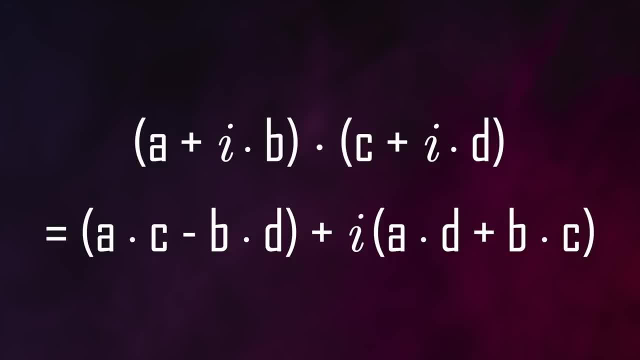 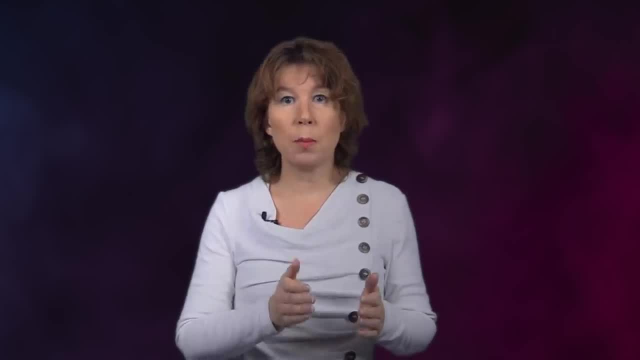 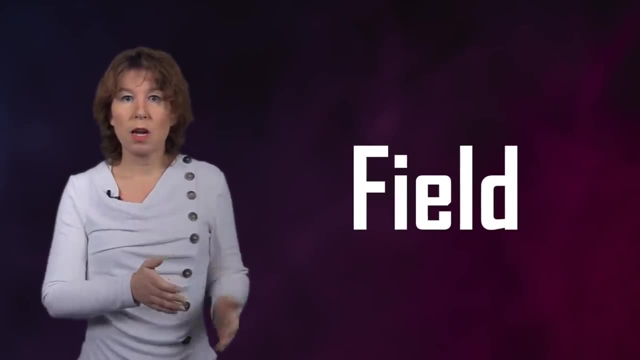 can work out by taking into account that the square of i is minus one. Two complex numbers can be added like they were vectors, but the multiplication law makes them different. Complex numbers are, to use the mathematical term, a field like the real numbers. They have a rule both for. 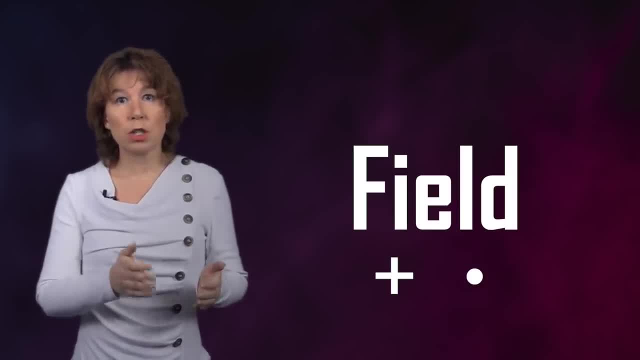 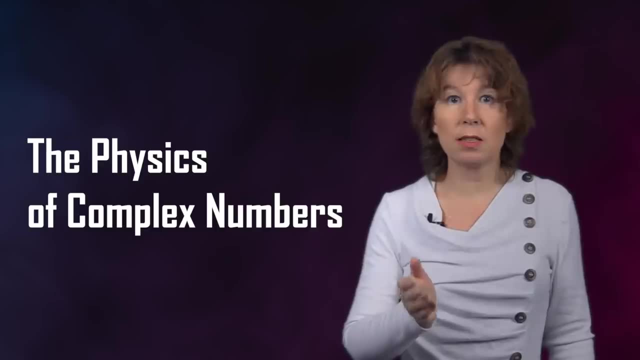 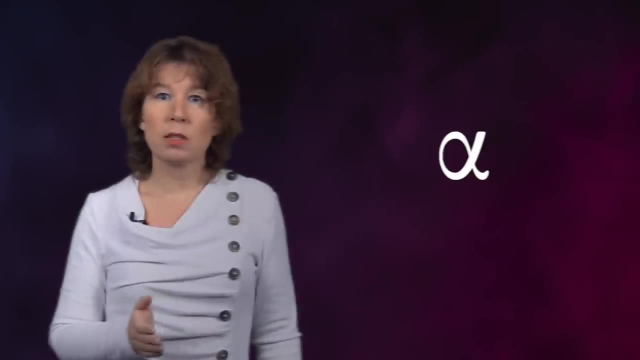 addition and for multiplication. They are not just like that two-dimensional grid. We use complex numbers in physics all the time because they are extremely useful. They are useful for many reasons, but the major reason is this: If you take any real number, 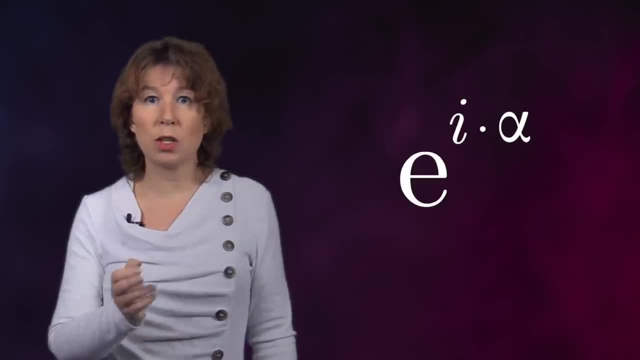 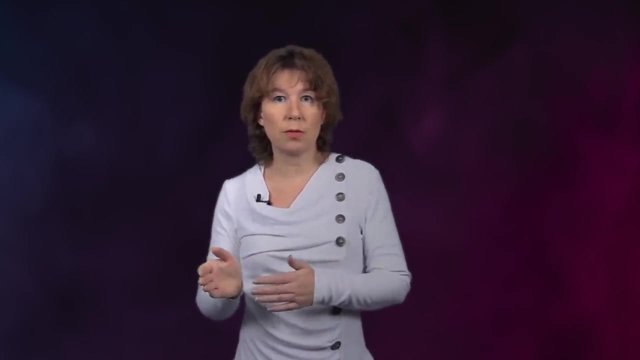 let's call it alpha. multiply it with i and put it into an exponential function, you get e to the i alpha. In the complex plane this number, e to the i alpha, always lies on a circle of radius one around zero. As you increase alpha, you'll go around that circle. Now, if you, 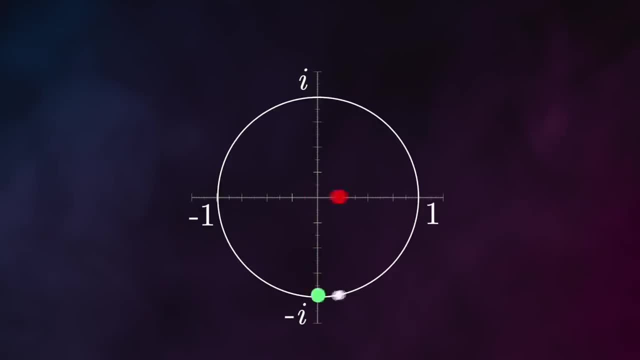 look only at the real or imaginary part of that circular motion, you'll get an oscillation. And indeed this exponential function is the sum of a cosine, and i times a sine function. Here's the thing: If you multiply two of these complex exponentials, say one with alpha and one, 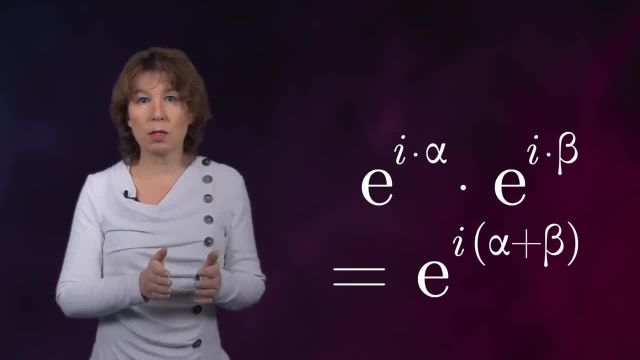 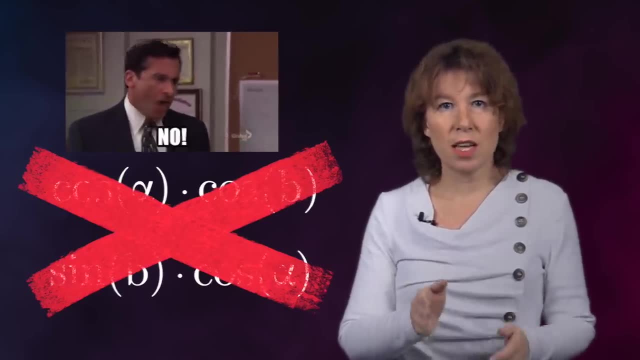 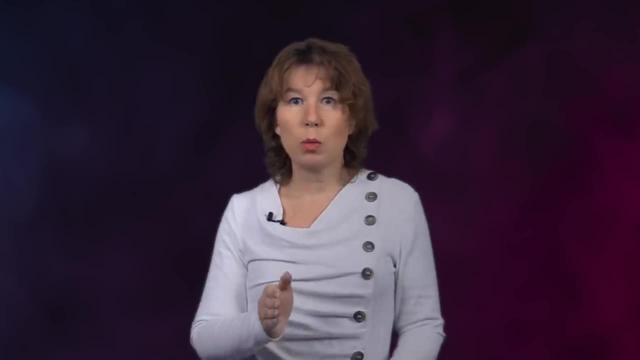 with beta, you can just add the exponents. But if you multiply two cosines or a sine with a cosine, that's a mess. You don't want to do that. That's why in physics we do the calculation with the complex numbers and then at the very end we take either the real or the imaginary. 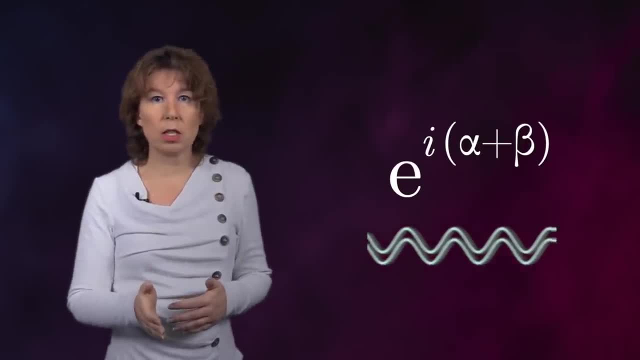 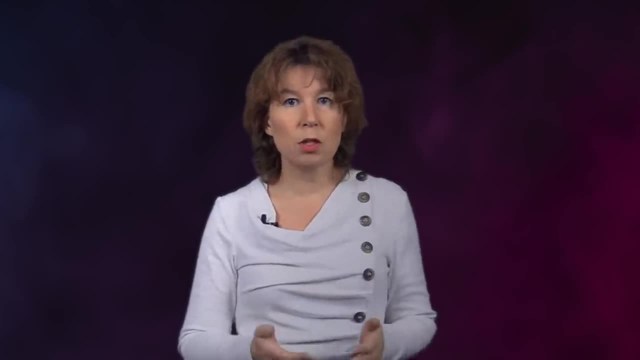 part. Especially when we describe electromagnetic radiation, we have to deal with a lot of oscillations, and complex numbers come in very handy, But we don't have to use them. In most cases we could do the calculation with only real numbers. It's just cumbersome- With the exception of quantum mechanics, to which we'll get in a moment. 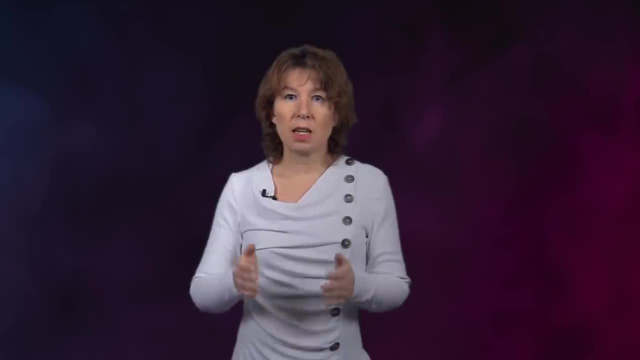 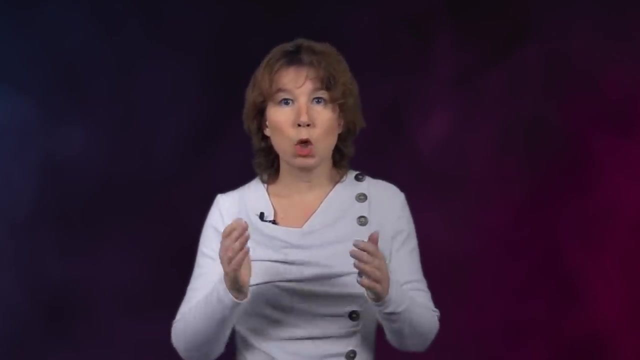 the complex numbers are not necessary And, as I have explained in an earlier video, it's only if a mathematical structure is actually necessary to describe observations we can say they exist in a scientifically meaningful way. For the complex numbers in non-quantum physics that's not the case. They're not necessary. 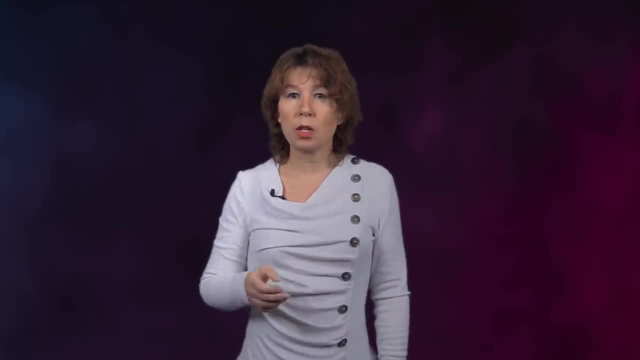 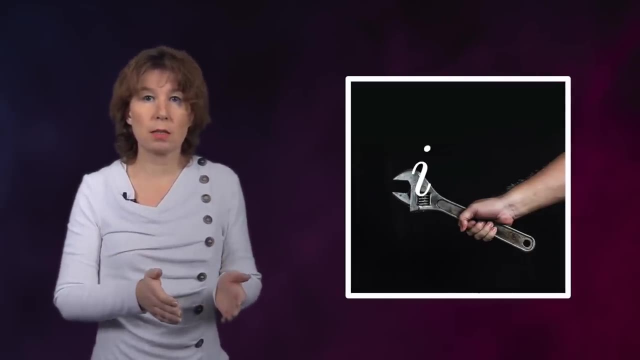 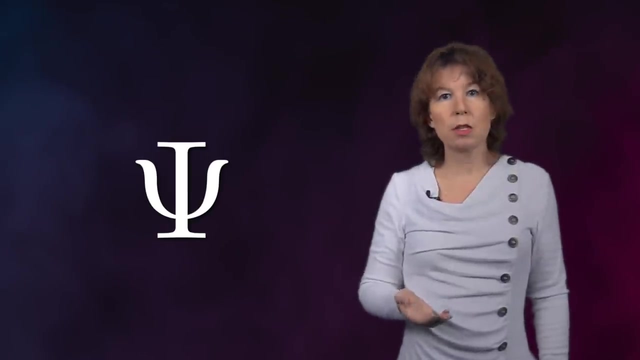 So as long as you ignore quantum mechanics, you can think of complex numbers as a mathematical tool and you have no reason to think they physically exist. Let's then talk about quantum mechanics. In quantum mechanics we work with wave functions, usually denoted psi. 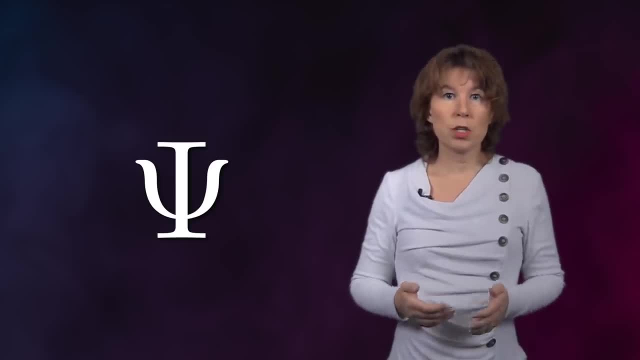 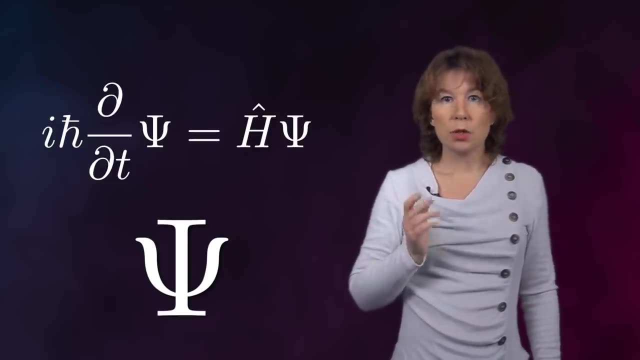 i, which are complex-valued, And the equation that tells us what the wave function does is the Schrödinger equation. It looks like this: You'll see immediately. there's an i in this equation, which is why the wave function. 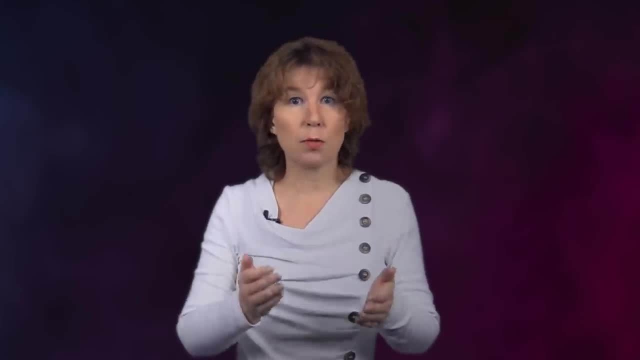 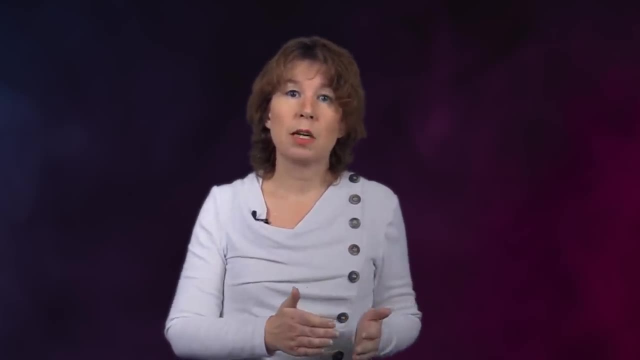 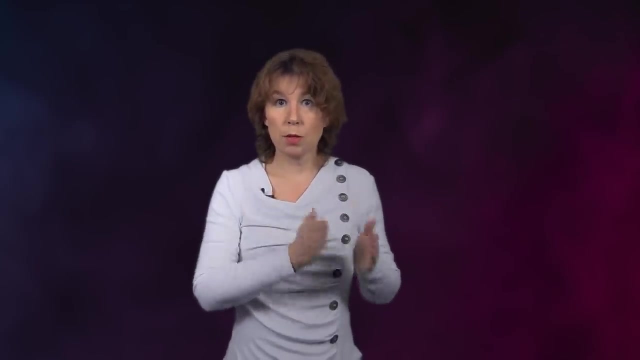 has to be complex-valued. However, you can of course take the wave function and this equation apart into a real and an imaginary part. Indeed, one often does that if one solves the equation numerically. And I remind you that both the real and the imaginary part 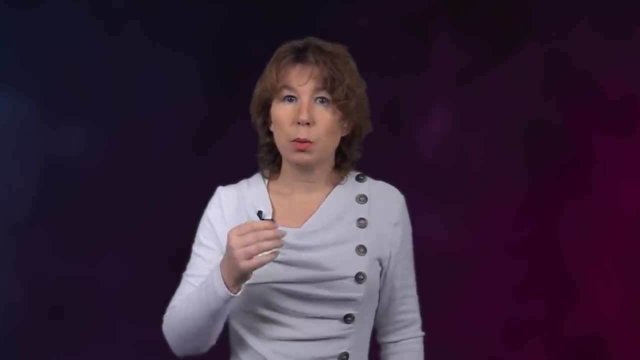 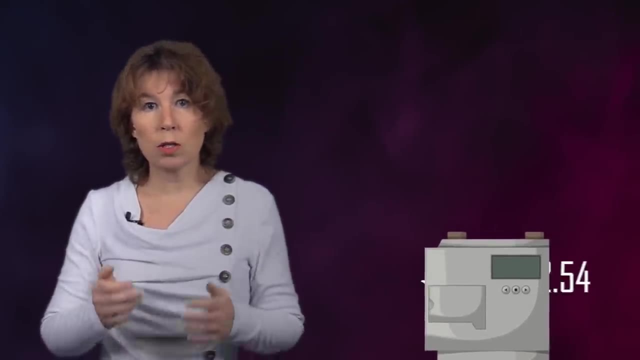 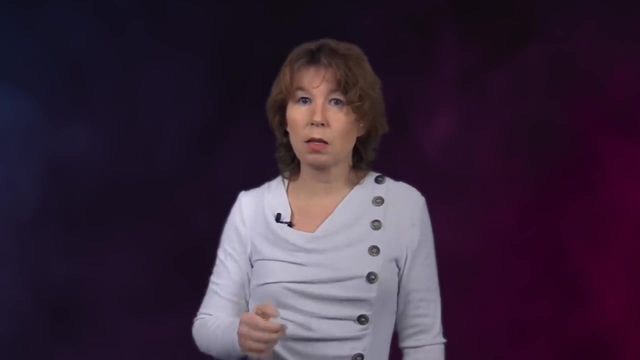 of a complex number are real numbers. Now if we calculate a prediction for a measurement outcome in quantum mechanics, then that measurement outcome will also always be a real number. So it looks like you can get rid of the complex numbers in quantum mechanics by splitting. 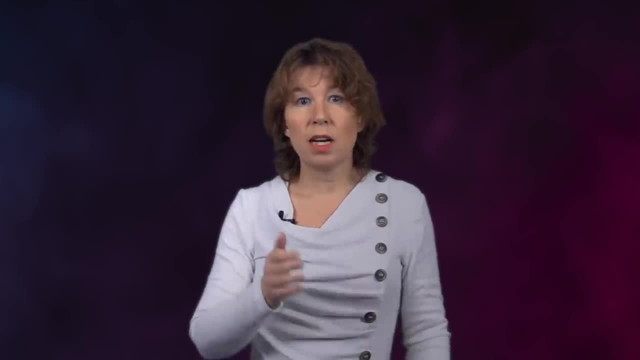 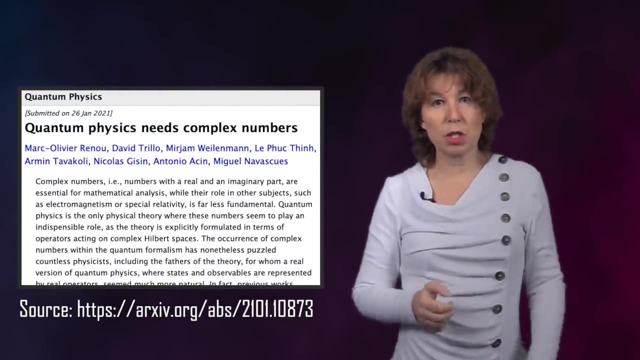 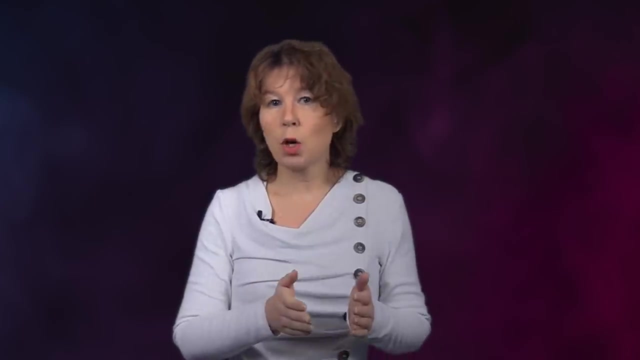 the equation into a real and an imaginary part, and that will never make a difference for the result of the calculation. This finally brings us to the paper I mentioned in the beginning. What I just said about decomposing the Schrödinger equation is, of course, correct, but that's not what they looked at in the 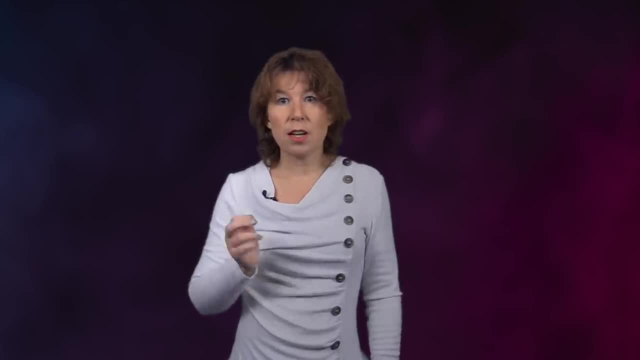 paper. That would be rather lame. Instead, they ask: what happens with a wave function if you have a system that's composed of several parts? In the simplest case, that would be several particles In normal quantum mechanics. each of these particles would have a function that is composed of several parts. In the simplest case, that would be several particles In normal quantum mechanics. each of these particles. 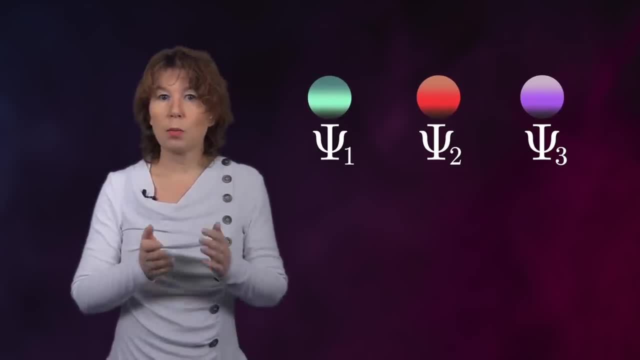 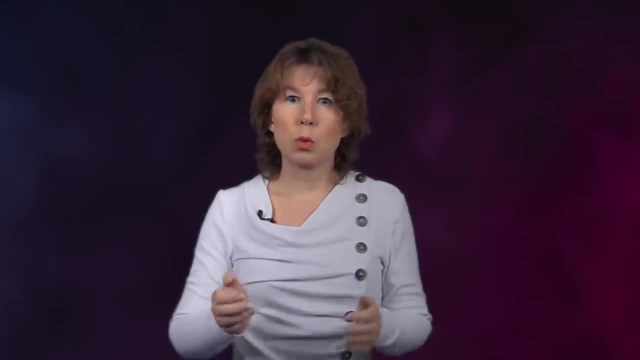 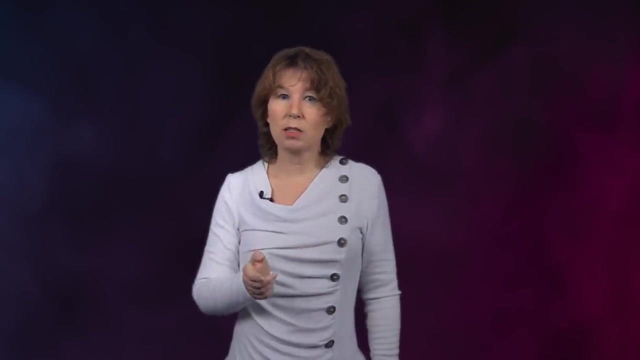 has a wave function that's complex-valued, and from these we construct a wave function for all the particles together, which is also complex-valued. Just what this wave function looks like depends on which particle is entangled with which. If two particles are entangled, 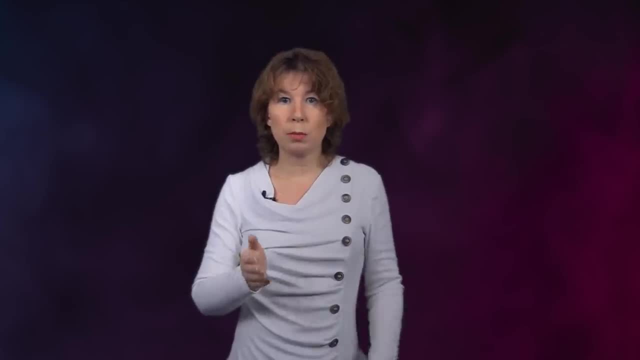 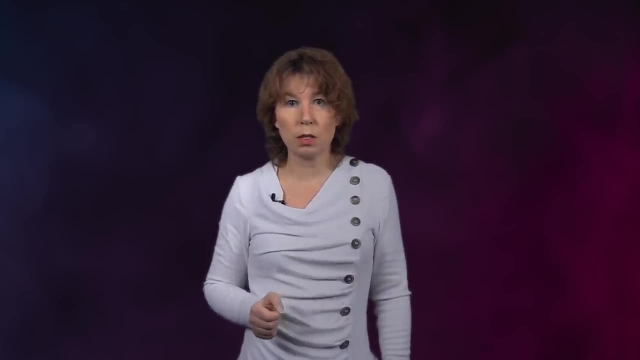 this means their properties are correlated, and we know experimentally that this entanglement correlation is stronger than what you can do without quantum theory. The question which they look at in the new paper is then whether there are ways to entangle particles in the 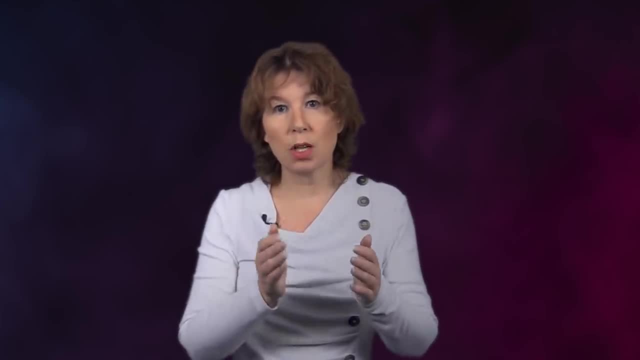 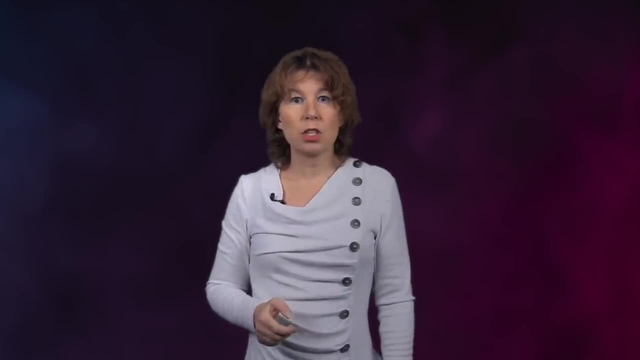 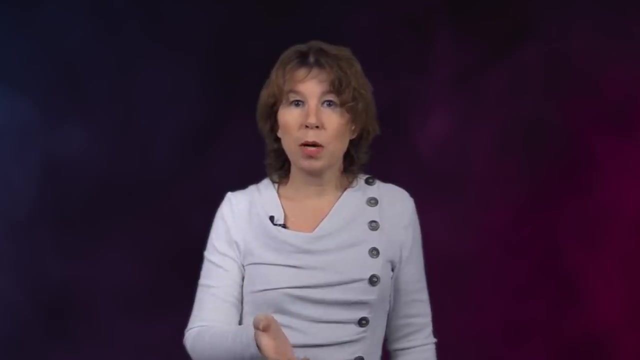 normal complex quantum mechanics that you cannot build up from particles that are described entirely by real-valued functions. Previous calculations showed that this could always be done if the particles came from a single source, But in the new paper they look at particles from two independent sources and claim that there are cases which you can't. 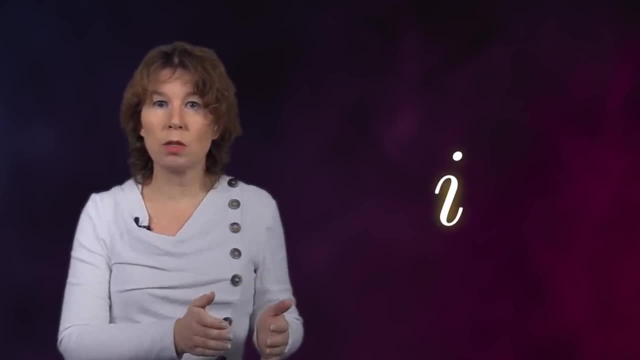 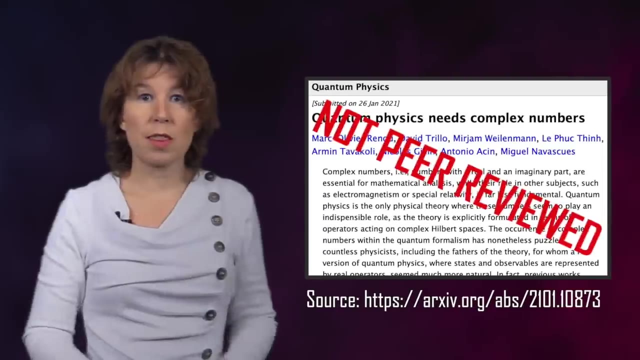 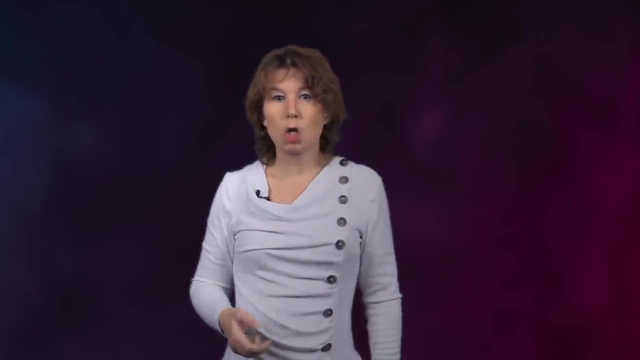 reproduce with real numbers only. They also propose a way to experimentally measure this specific entanglement. I have to warn you that this paper has not yet been peer-reviewed, so maybe someone finds a flaw in their proof, But assuming their result holds up, this means if the experiment which they propose finds: 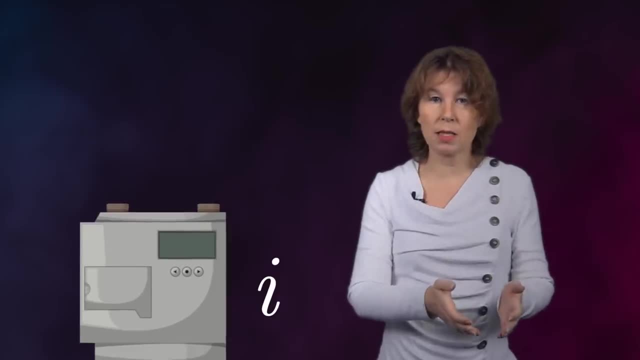 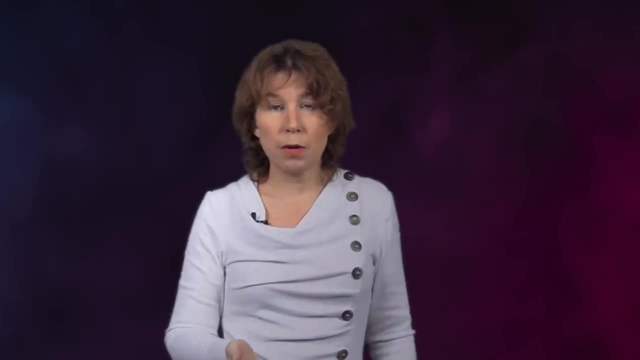 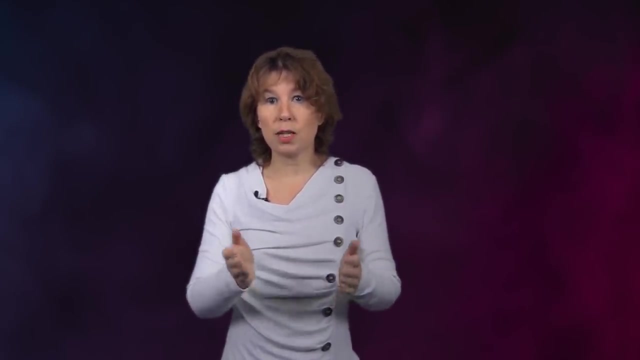 the specific entanglement predicted by complex quantum mechanics, then you know you can't describe observations, And it would then be fair to say that complex numbers exist. So this is why it's cool They've figured out a way to experimentally test if complex numbers exist Well, kind of, Here's the fine print. This conclusion only applies if you want the purely real-valued theory to work the same way as normal quantum mechanics, If you are willing to alter quantum mechanics so that it becomes even more non-local than. 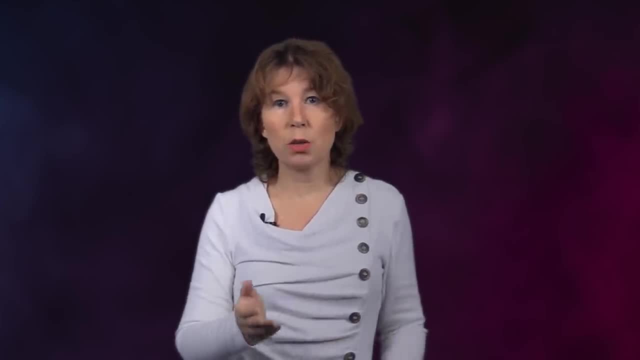 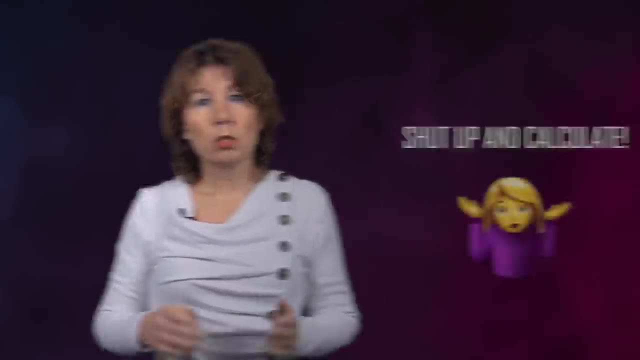 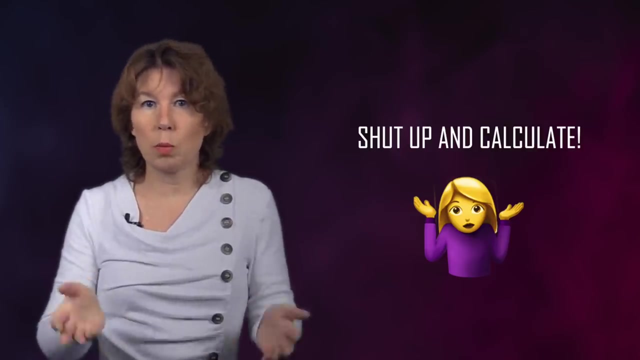 it already is, then you can still create the necessary entanglement with real-valued numbers. Why is it controversial? Well, if you belong to the shut-up-and-calculate camp, then this finding is entirely irrelevant, Because there's nothing wrong with complex numbers in the 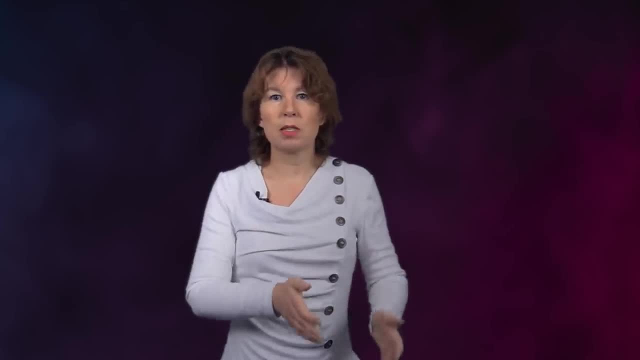 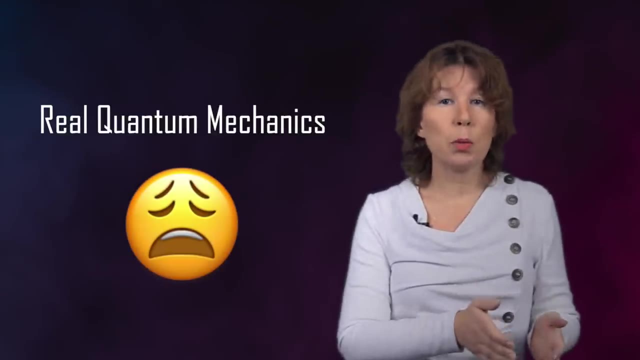 first place. So that's why you have half of the people saying what's the point or why all the fuss about it, if you, on the other hand, are in the camp of people who think there's something wrong with quantum mechanics because it uses complex numbers. 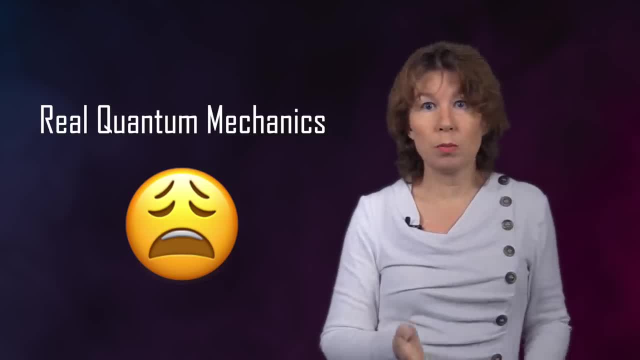 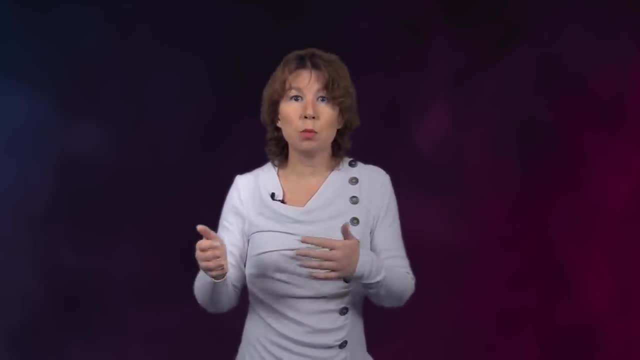 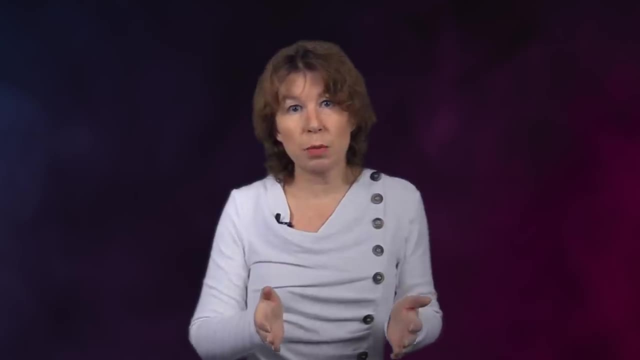 that we can never measure, then you are now caught between a rock and a hard place. Either embrace complex numbers or accept that nature is even more non-local than quantum mechanics already is. Or, of course, it might be that the experiment will not agree with the predictions of quantum mechanics, which would be the most exciting. 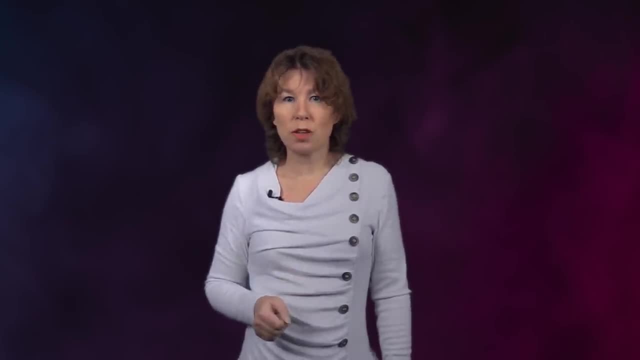 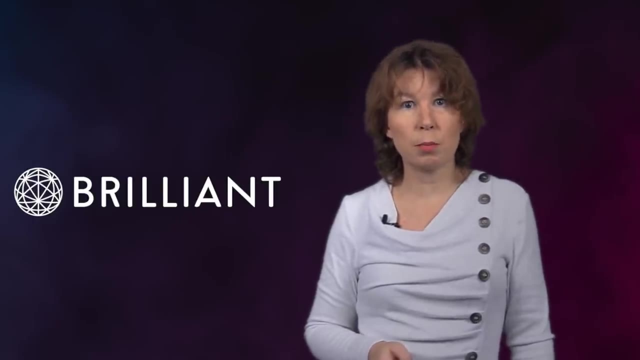 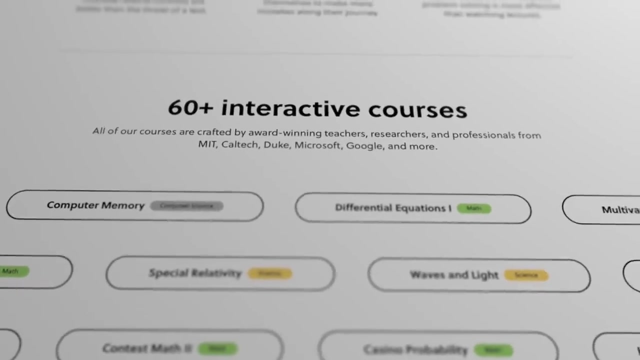 of all possible outcomes. Either way, I'm sure that this is a topic we'll hear about again. This video was sponsored by Brilliant, which is a website and app that offers interactive courses on a large variety of topics in science and mathematics. If you want to really understand, 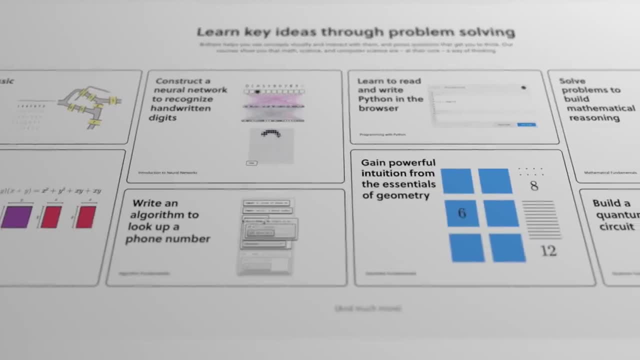 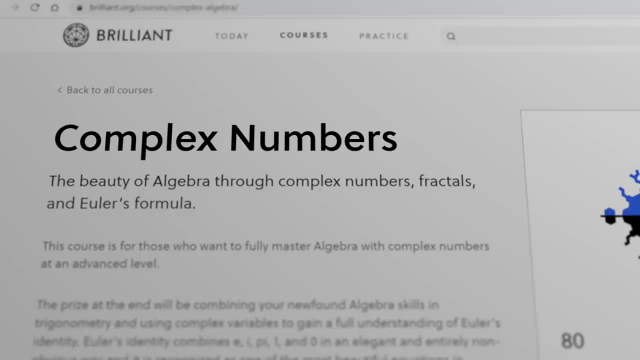 complex numbers and their role in quantum mechanics. Brilliant is a great starting place for that. To get more background on this video's topic, have a look, for example, at their courses on complex numbers. Thanks for watching. Thanks for watching. See you next week. Subtitles by the Amaraorg community.